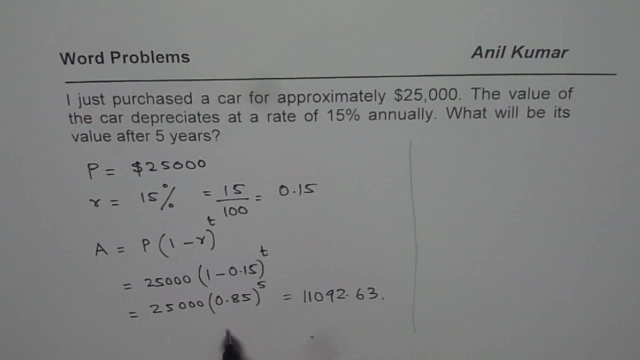 In case you haven't learned this. in that case, how are you going to solve the question Now that, In that case, you should- You should be making a table of values, You can say: let this be the original cost, which. 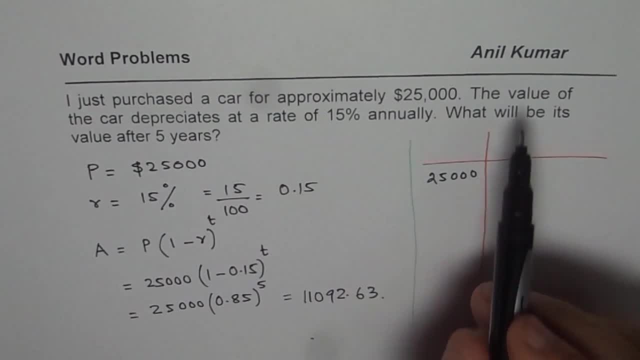 is, let us say, 25,000,. right Now it says every year: so if t after one year, what will happen? So every year, what happens? So after one year it actually reduces by 15%, 15% of its value. You get the point. The value of the car depreciates at a rate. 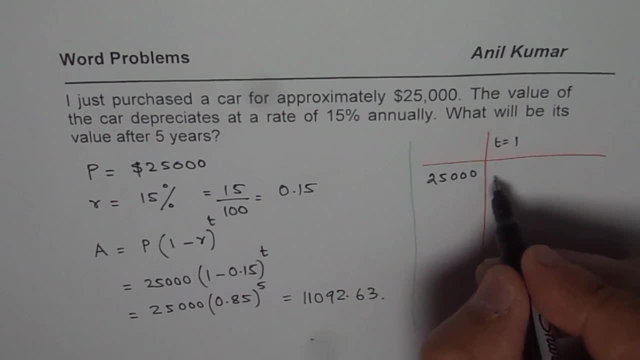 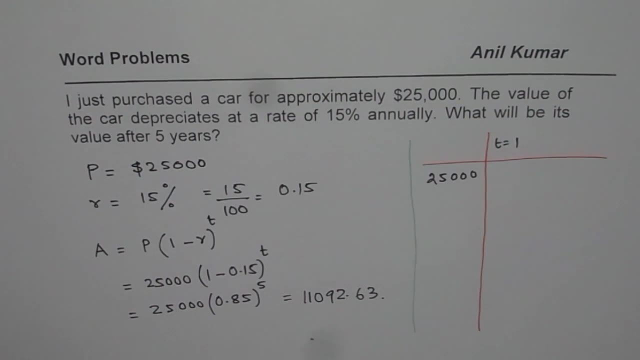 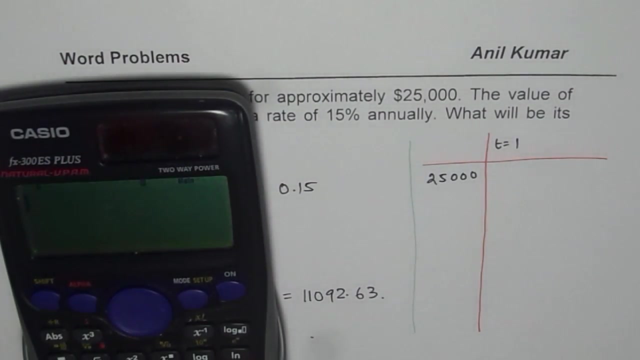 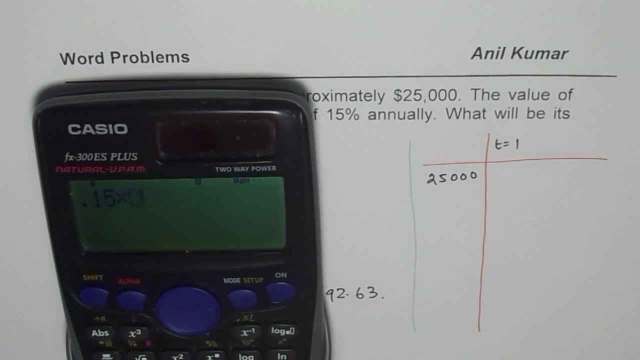 of 15% annually. right, You can get this. You can find 15% of this amount and then take away that amount, right, So we get 15% of. So that means 0.15 of that amount. So 15% of 25,000 is equals to 3750, right, So that. 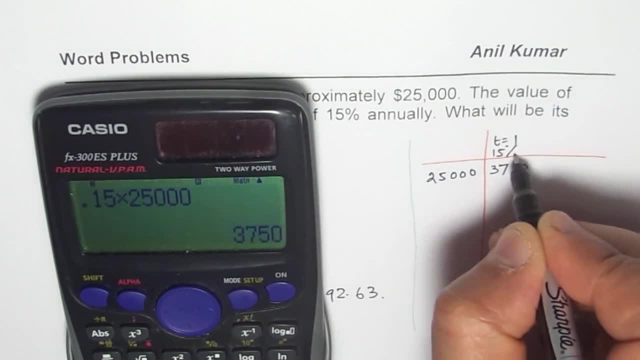 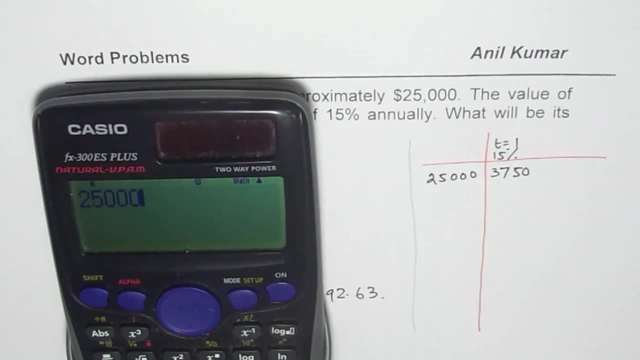 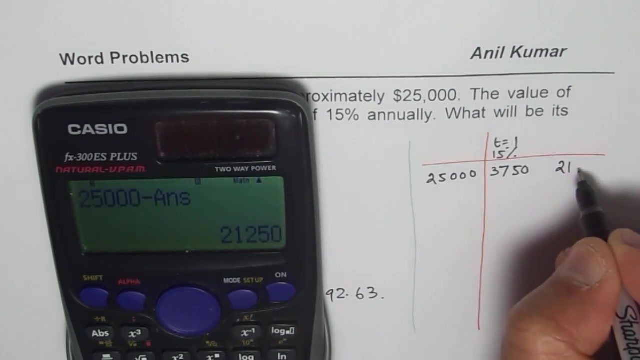 is 1550.. Okay, Here we go, we're done. So this whole thing. Okay, percent. right now, that value should be deducted from 25 000, so we get 25 000. take away 3750, which is our answer is equal to. so what you get is 21 250 dollars, right? so what i'm trying to tell you? 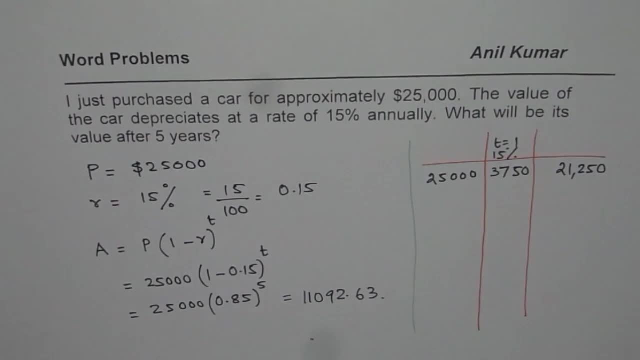 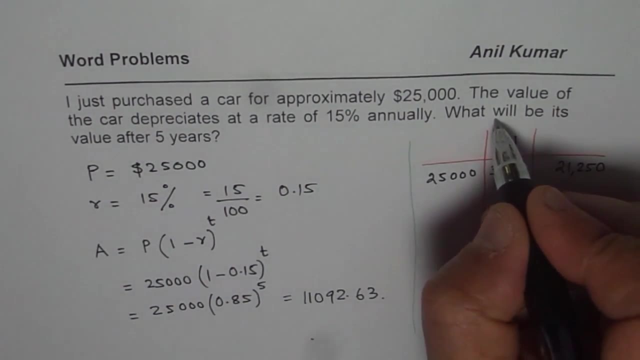 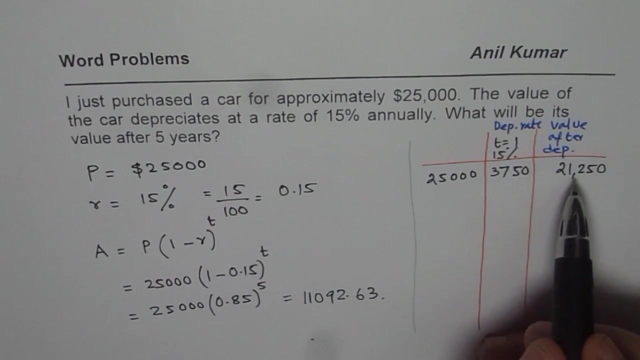 you can make a table like this correct, where one column of the table will be the deduction or depreciation right depreciation rate per year. so that is the and that is the value after depreciation, correct? so this will be the amount given here. let me call this as the amount. 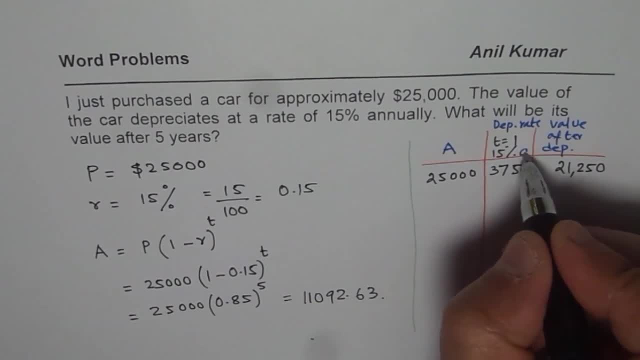 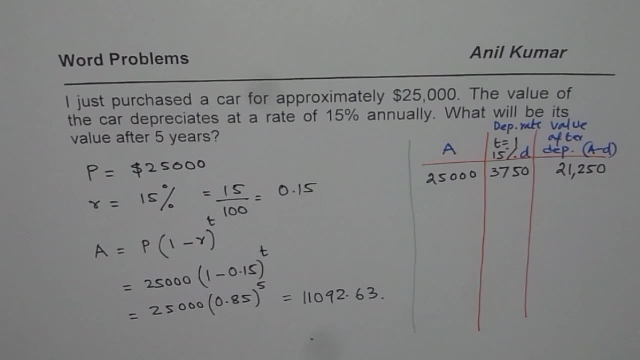 right. so the amount minus- let us say this- is depreciation, so this column will be a minus d. you get my point right. so you can continue this column and then find your answer. so that is the alternate way of solving this question. so in case you don't know what this formula is, then you can apply this: 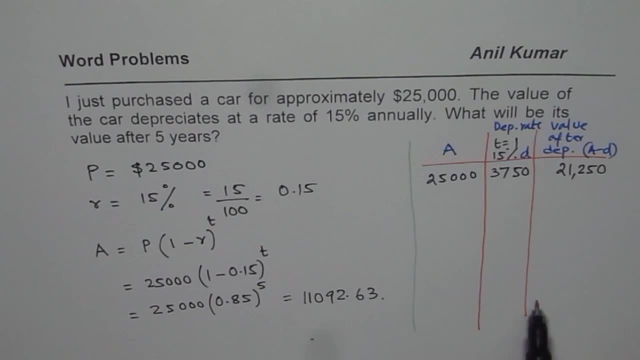 technique to answer the question right. i hope that helps. now. this particular list of videos is for students who have done math long time back and now they are again getting back to the college, so it is for them. therefore, they might have forgotten some things. i hope these techniques 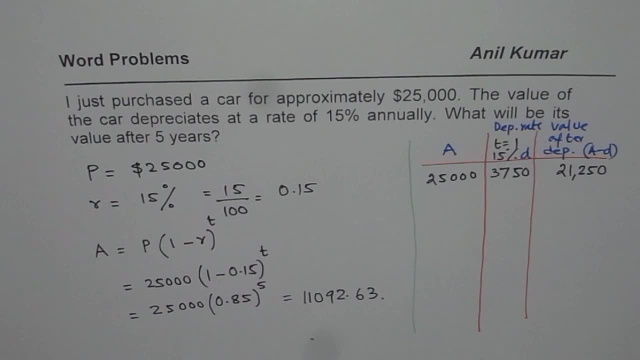 help them to get the right answers. thank you and all the best. 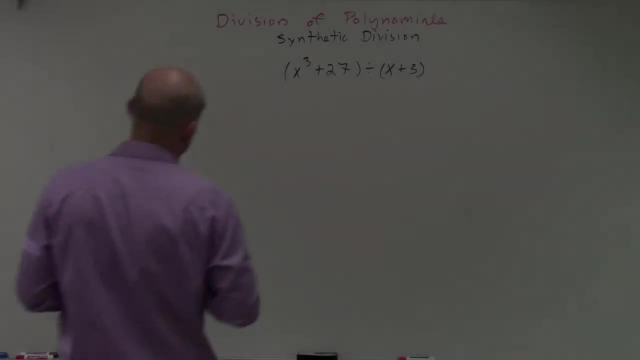 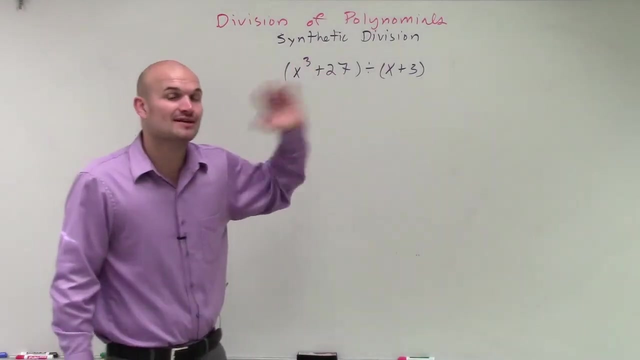 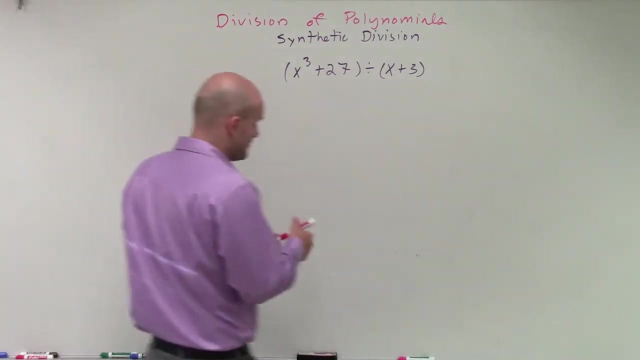 Okay, welcome. So I chose this problem because you can see I have a lot of missing terms. I go from x cubed down to 27.. So when we're writing the synthetic division problem, we need to make sure we also include the place value for x squared and x. But the main first. 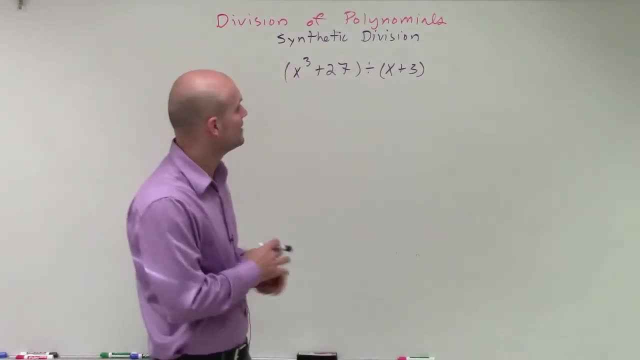 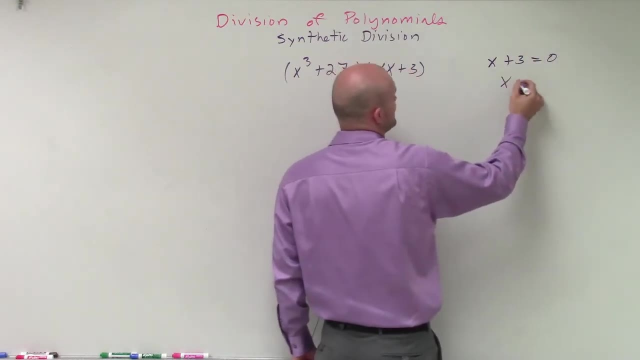 thing we always want to look at as our divisor, make sure that it's linear and in the form of binomial, which in case it is, So, therefore, we can just take it and say x plus 3 equals 0 and then say: all right, well, that means x is going to equal negative 3, as I solve, 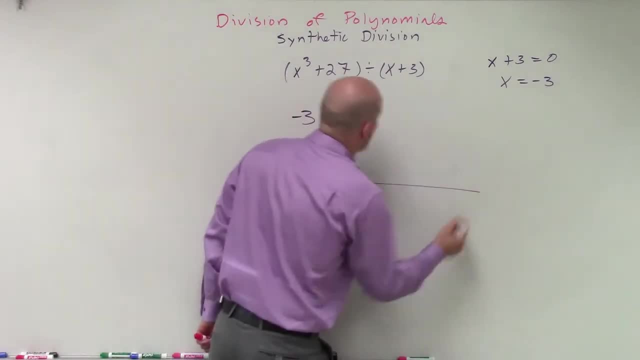 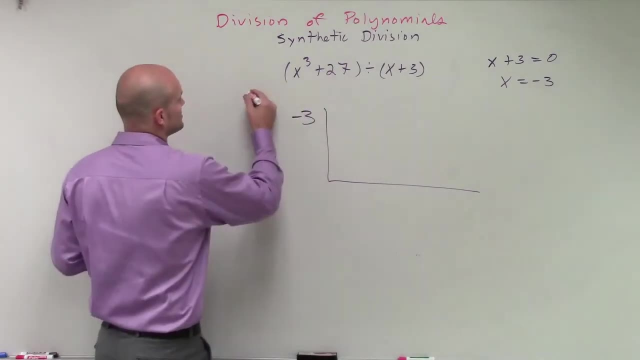 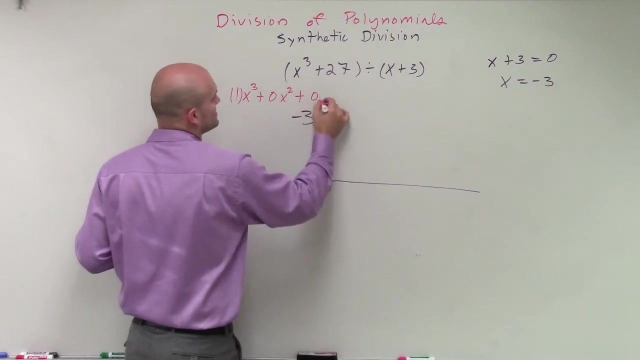 for it, right? So that's going to be on my outside. Then I know I need to take the coefficient of each one of my terms And remember. I can rewrite this by including all my values of saying it's x to the cube, which would be like 1x cubed plus 0x squared plus 0x plus. 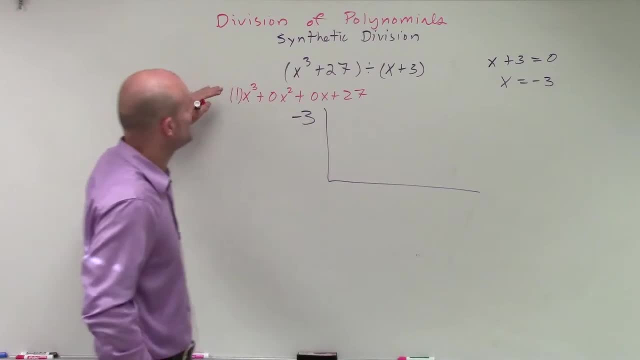 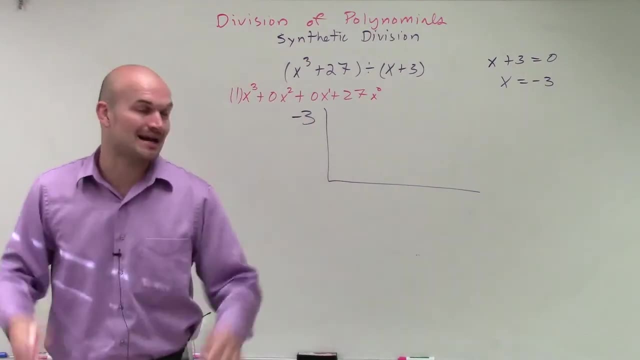 27.. And we need to make sure we use that value so that we have it in descending order, which this could be like an x to the first And that could be an x to the 0.. All right, I'm getting a little bit way, kind of beyond. 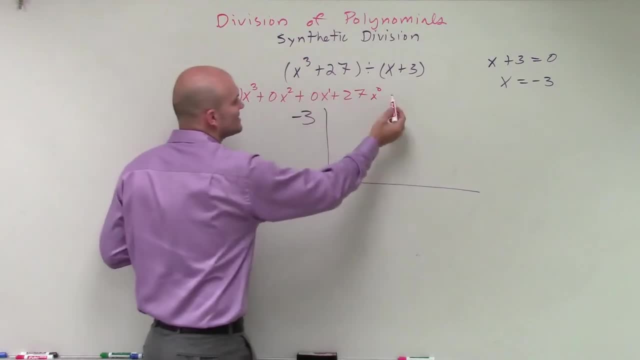 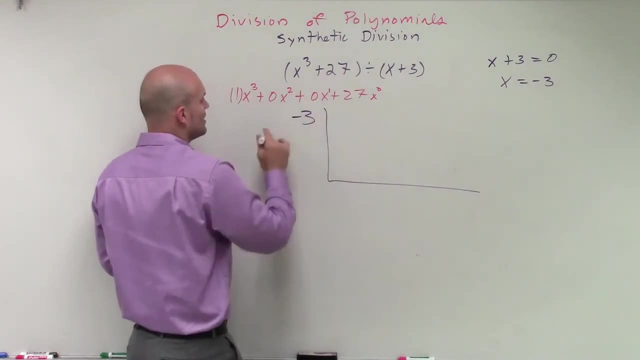 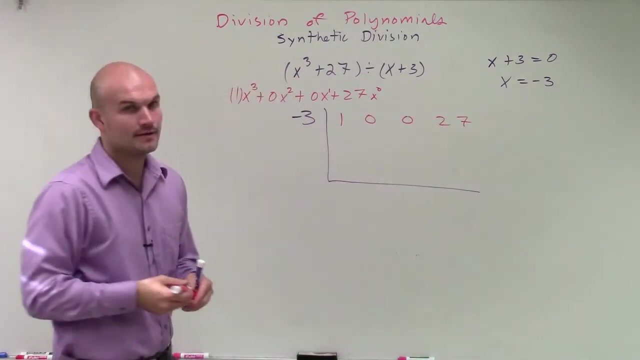 what we need to. But you can see that this goes down. My variables go down in descending order. We need to make sure we include all of our place values. So the leading coefficients for each one of my terms and my constant are going to be 1, 0, 0, 27.. So now let's go and